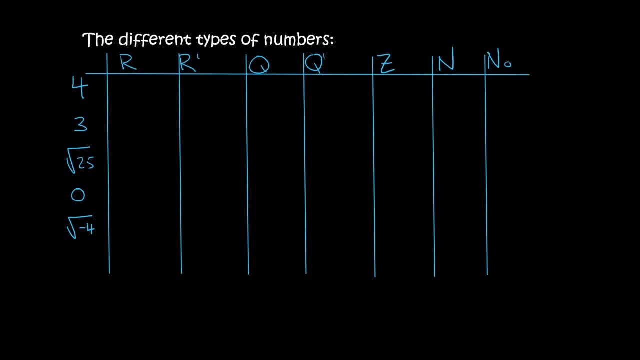 Hello everyone. so in this lesson I'm going to show you the different kinds of numbers. So at the top here I've got all these different letters. Now let's quickly define them. So R stands for real, R with a little line means not real or non-real. Q stands for rational. 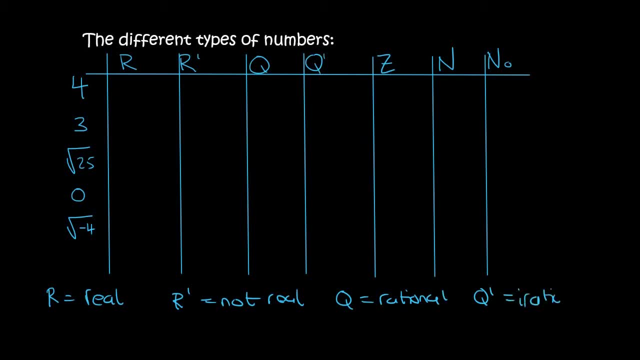 Q with a line is irrational, which means not rational. Z stands for integer, N stands for natural N with a little zero stands for whole numbers. So the number four. is it real? Can you see it? Yes, So it can't be this one, so I'm going to put a little x there. 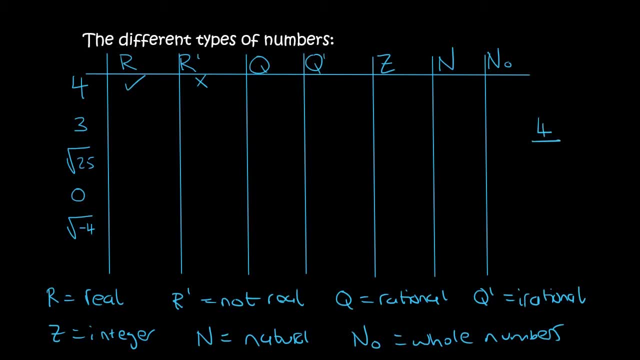 Rational is any number that can be written as a fraction. So four is the same as four over one. So yes, it is rational, which means it's not irrational. Integers are the numbers like minus three, minus two, minus one, zero one, two, three and so on and so on. It's the numbers. 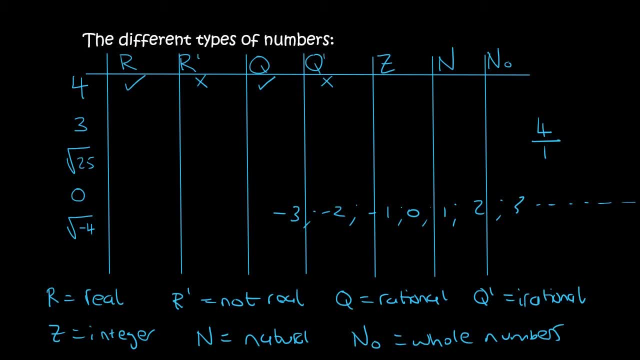 that can be negative and positive, but they must be complete. They mustn't be numbers like minus one comma seven, eight, three, Not that. So the number four is an integer Natural numbers. Now if I asked you to start counting, you would start by saying one, two, three, four. So four is. 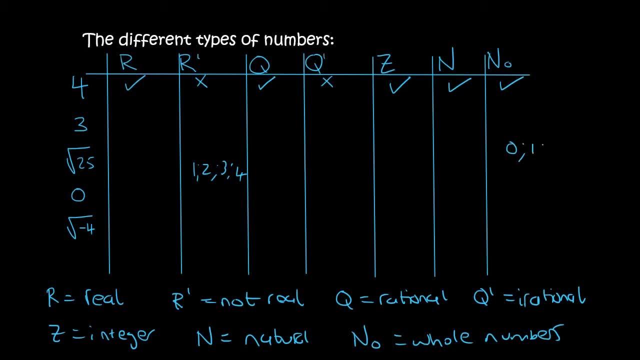 also a whole number. Whole numbers start at zero. So zero one, two, three, four. The number three is obviously they're going to be the same as the number four. There's no major difference between them. Square root of 25.. Now students panic when they see this. but guys, square root of 25,. 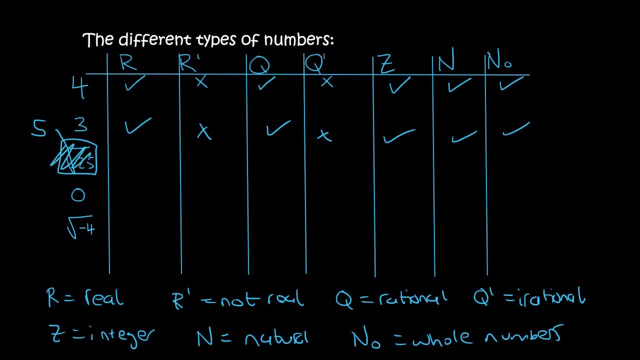 what is that? That is five, And so we can actually cross this out and pretend that it's a five. Now, if it's a five, then it follows the same as three and four. The number zero is real Rational, because zero is the same as zero over one, So you can write it as a fraction. 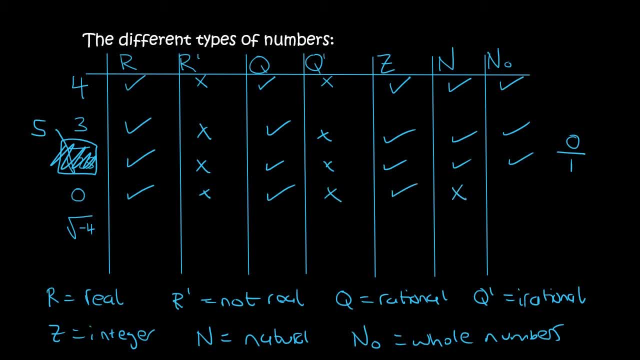 It is an integer. It's not a natural number, because when you count, naturally, you start at one. It is a whole number, though, because you start at zero. If you type this on your calculator, try that quickly. What you'll see is that you're going to get an error. 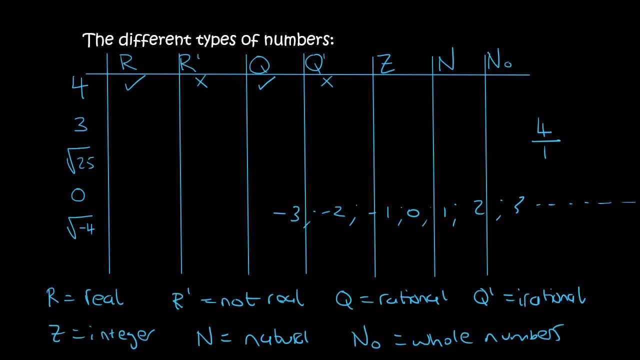 that can be negative and positive, but they must be complete. They mustn't be numbers like minus one comma seven, eight, three, Not that. So the number four is an integer: Natural numbers. Now if I asked you to start counting, you would start by saying one, two, three, four. So four is a. 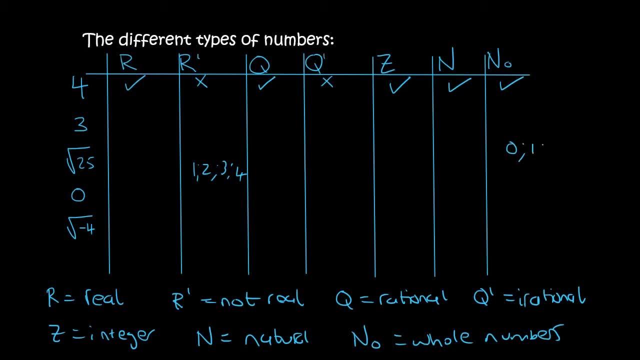 whole number. Whole numbers start at zero. So zero one, two, three, four. The number three is obviously. they're going to be the same as the number four. There's no major difference between them. Square root of 25.. Now students panic when they see this. but guys, square root of 25,. 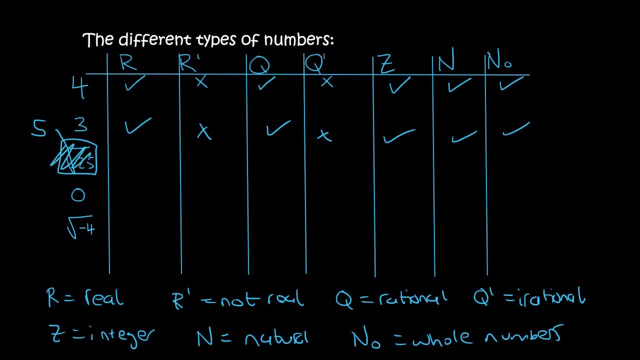 what is that? That is five, And so we can actually cross this out and pretend that it's a five. Now, if it's a five, then it follows the same as three and four. The number zero is real Rational, because zero is the same as zero over one, So you can write it as a fraction. 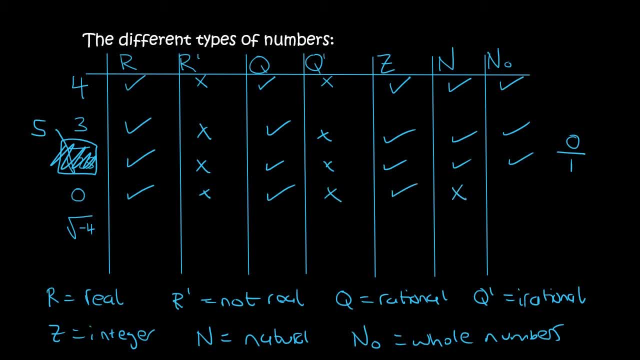 It is an integer. It's not a natural number, because when you count, naturally, you start at one. It is a whole number, though, because you start at zero. If you type this on your calculator, try that quickly. What you'll see is that you're going to get an error. 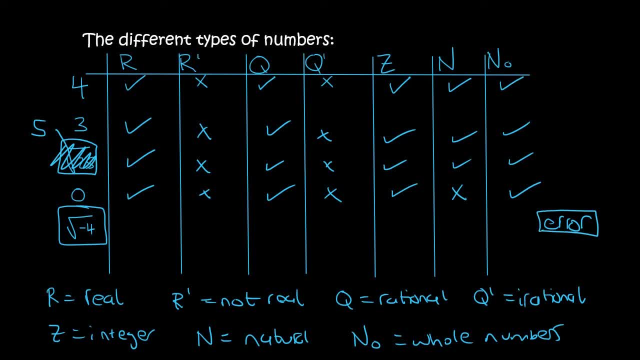 Now you get two different kinds of errors. When it's because of a square root, then we call that non real or not real. So it's this one, which means it can't be that one And it can't be any of the others. I want to add one more. 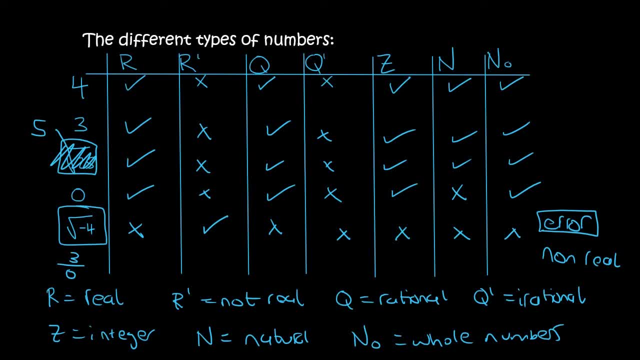 If we have the number three over zero, go ahead, type that in on your calculator and you're going to get an error again. Oh, I should have added another column over here. I do apologize, called undefined. When you have an error due to a zero underneath, then that's called undefined. and 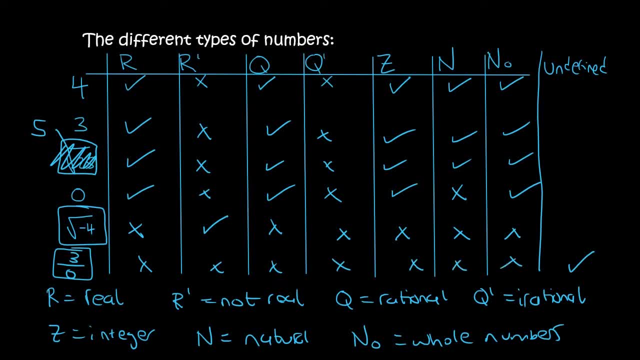 it can't be any of the other ones Undefined. think of it as when the zero is underneath, You can have a zero on top, like that. That just gives you zero, So that's okay, But what you don't want is a zero underneath. Here's another set of numbers. If you type in pi on your calculator. 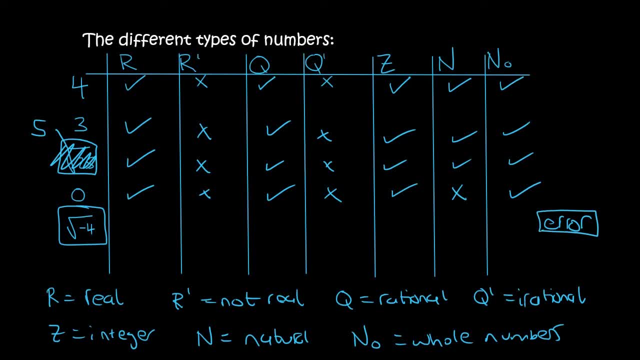 Now you get two different kinds of errors. When it's because of a square root, then we call that non real or not real. So it's this one means it can't be that one and it can't be any of the others. I want to add one more. 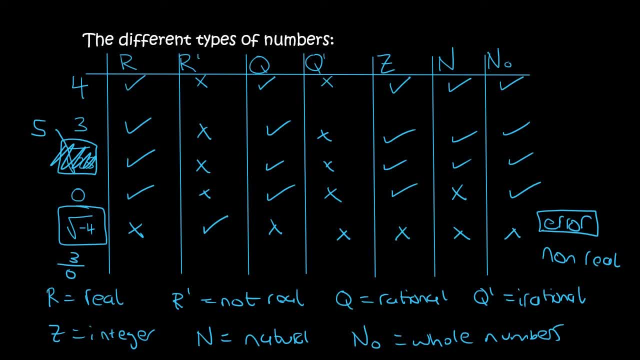 If we have the number three over zero, go ahead, type that in on your calculator and you're going to get an error again. Oh, I should have added another column over here. I do apologize. called undefined When you have an error due to a zero underneath. 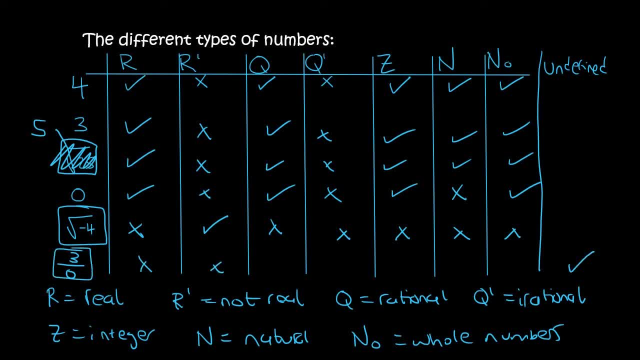 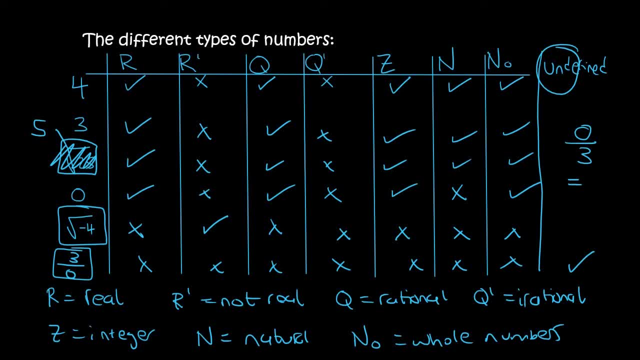 You can have a zero on top like that. That just gives you zero, So that's okay, But what you don't want is a zero underneath. Here's another set of numbers. If you type in pi on your calculator, you'll see that it's like 3.14, and then the numbers don't repeat. If the numbers do repeat, 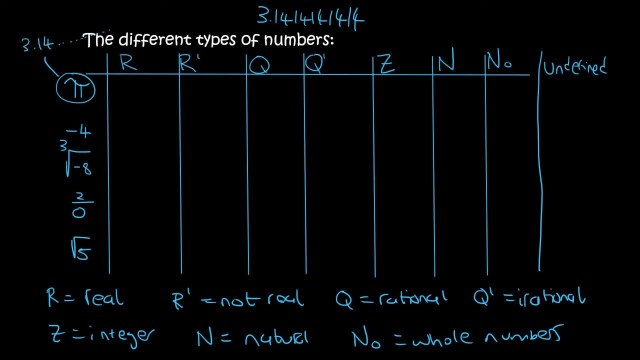 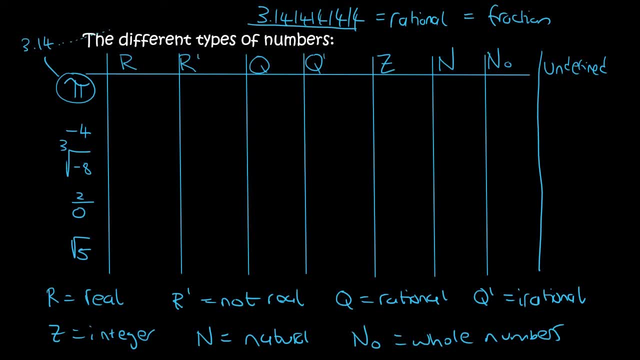 But pi, the digits do not repeat. So that is, oh, it's still a real number. Can you see pi? Yeah, I can see it. So it's a real number. It's not going to be rational, though It's going to be. 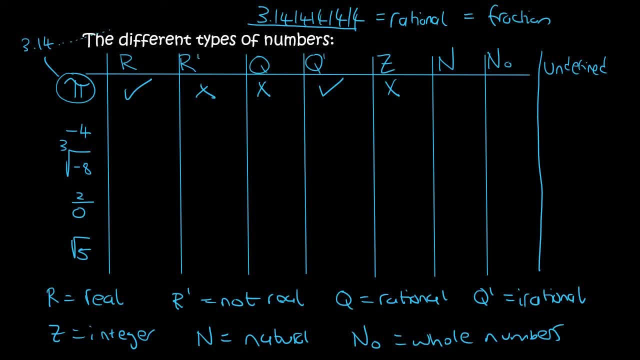 irrational. Is it an integer? No, because integers are whole, They are complete, Minus three, minus two, minus one zero, like that. Is it natural? No, If I count from one, two, three, I don't go one, two, three, three comma, one, four. No, I say one, two, three, four. Is it a? 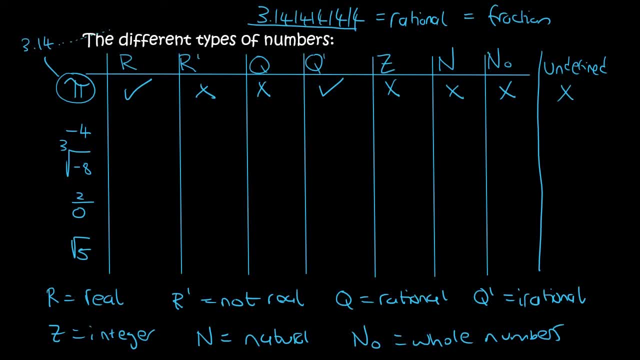 whole number? No, Is it undefined? No, it is defined: The number minus four. is it real? Yes, you can see it. Is it so? obviously it's not non-real. It is rational, because minus four is the same as minus. 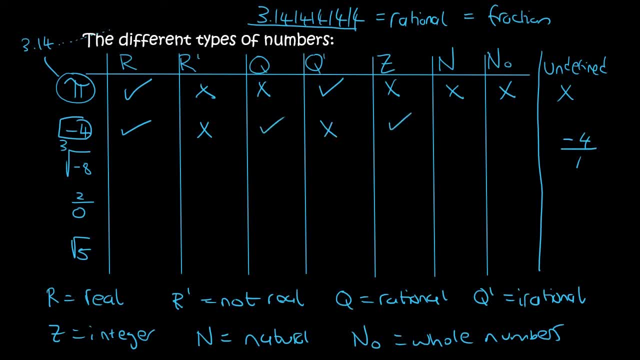 four over one, So it can't be that one. Is it an integer? Yes, it is, because it's minus four, minus three, minus two. Is it natural? No, you're not going to count that. if you were counting, 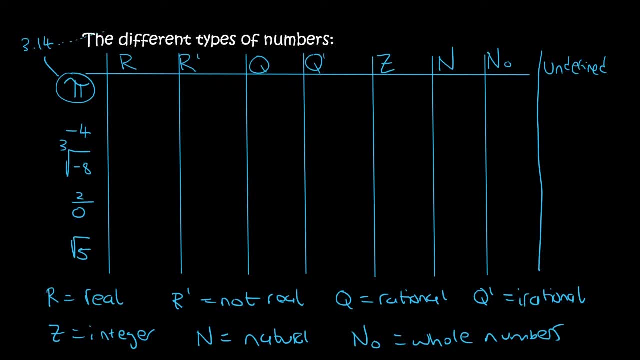 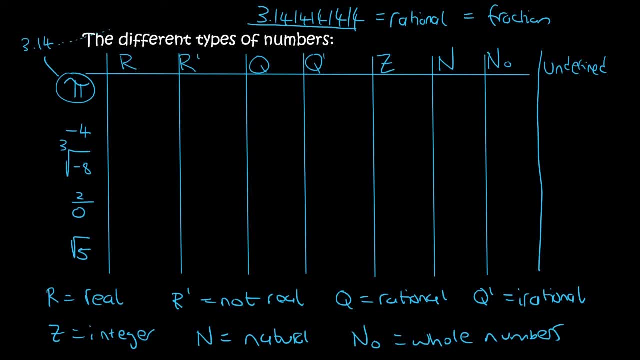 repeat, But pi, the digits do not repeat. So that is, oh, it's still a real number. Can you see pi? Yeah, I can see it. So it's a real number. It's not going to be rational, though It's going to be. 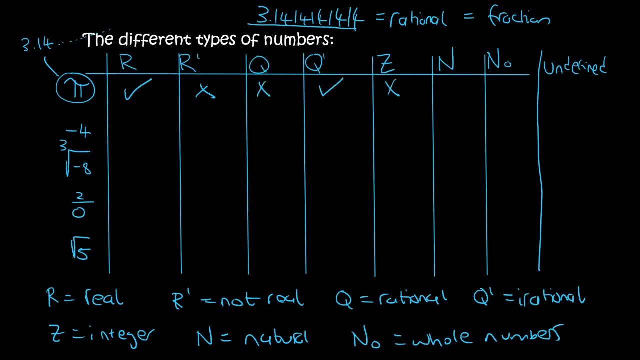 irrational. Is it an integer? No, because integers are whole, They are complete, Minus three, minus two, minus one zero, like that. Is it natural? No, If I count from one, two, three, I don't go one, two, three, three comma, one, four. No, I say one, two, three, four. Is it a? 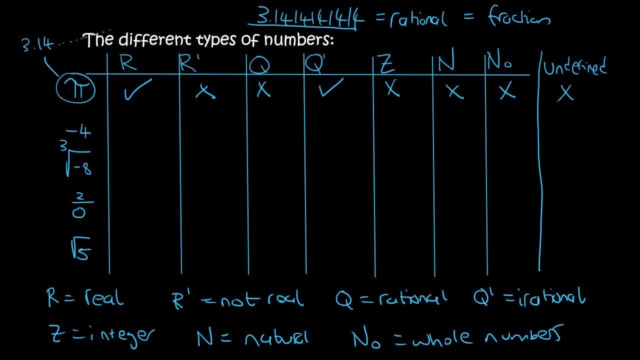 whole number? No, Is it undefined? No, it is defined: The number minus four. is it real? Yes, you can see it. Is it so? obviously it's not non-real. It is rational, because minus four is the same as minus. 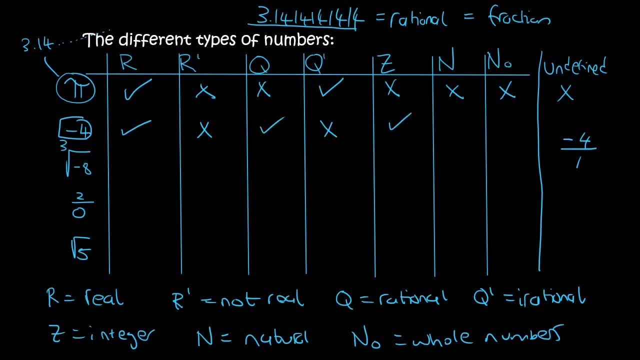 four over one, So it can't be that one. Is it an integer? Yes, it is, because it's minus four, minus three, minus two. Is it natural? No, you're not going to count that. if you were counting, 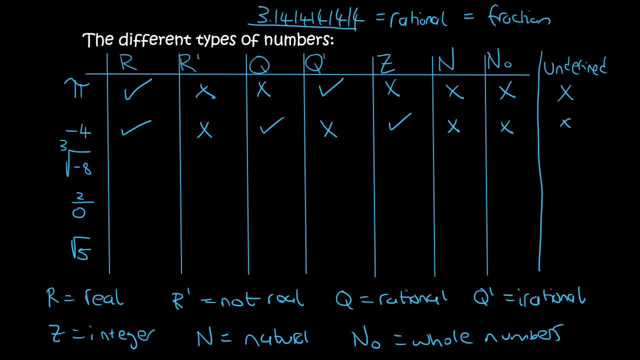 And is it a whole number? No, it's not And it's not undefined. If you type this on your calculator, you're not going to get an error. You only get an error when you have a negative inside a normal square root or any even number. 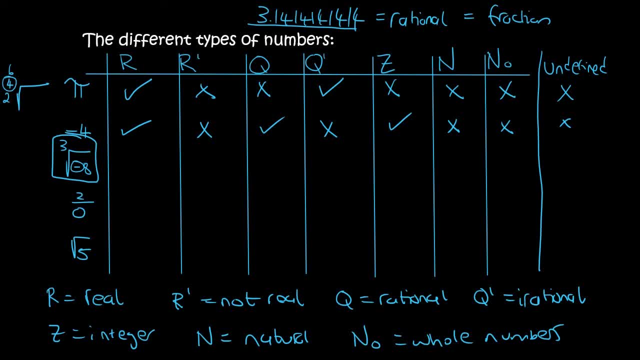 like four, six or two. So what I would say is: if you're in an exam, type it in on your calculator And if you get an error then obviously that's a problem. But with this one you wouldn't get. 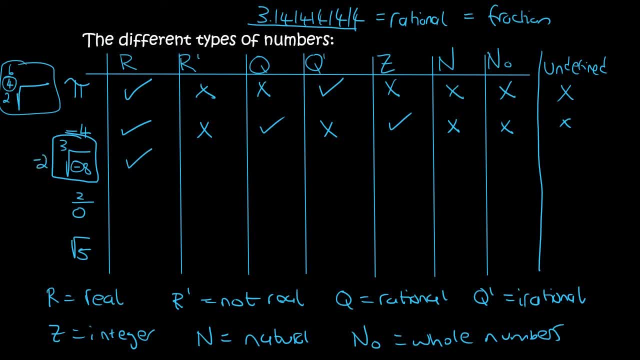 an error, You would get minus two. The number minus two is real, It's rational, It's an integer, but it's not natural. And it's none of these other ones: Two over zero. Type it in on your calculator, because if you're in a test you don't want to. 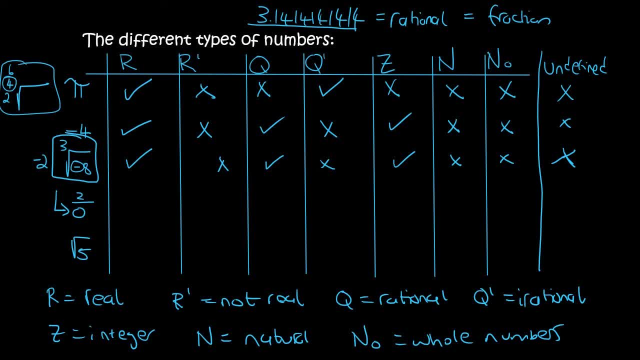 think: wait, can the zero be at the bottom or is it at the top? What did Kevin say? Guys, just type it in on the calculator and you're going to get an error. But that error is because of the zero that is underneath, And so it's undefined And that's all. All the others will not work. Square root. 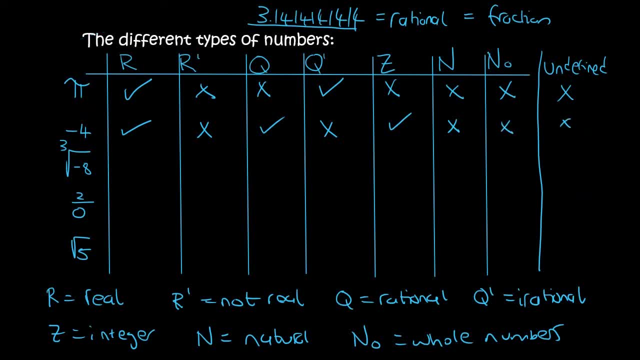 And is it a whole number? No, it's not And it's not undefined. If you type this on your calculator, you're not going to get an error. You only get an error when you have a negative inside a normal square root or any even number. 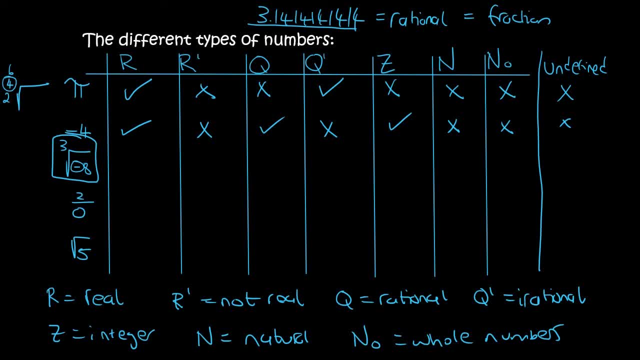 like four, six or two. So what I would say is: if you're in an exam, type it in on your calculator And if you get an error then obviously that's a problem. But with this one you wouldn't get an. 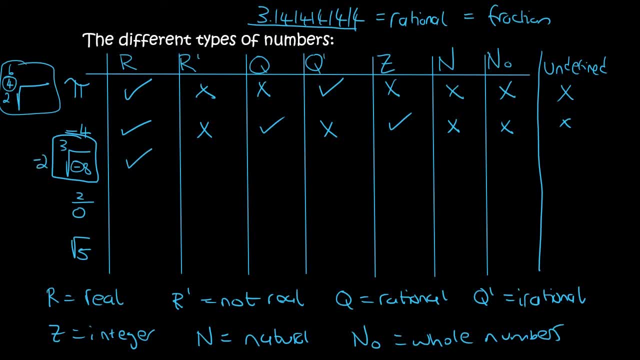 error, You would get minus two. The number minus two is real, It's rational, It's an integer, but it's not natural. And it's none of these other ones, Two over zero. Type it in on your calculator, because if you're in a test you don't want to. 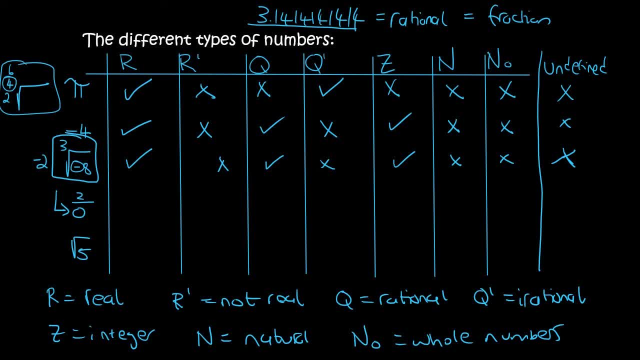 think: wait, can the zero be at the bottom or is it at the top? What did Kevin say? Guys, just type it in on the calculator and you're going to get an error. But that error is because of the zero that is underneath, And so it's undefined And that's all. All the others will not work. 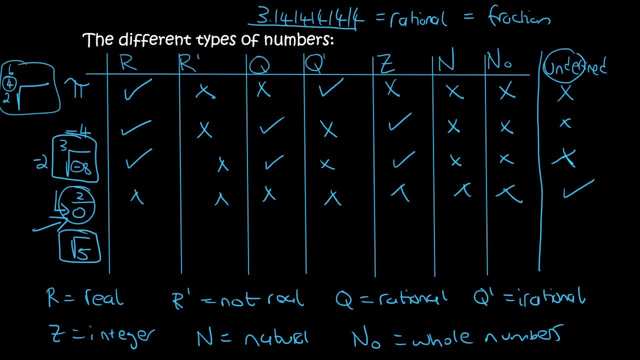 Square root five. Type it in on your calculator and you're going to get some weird. you're going to get something like two comma, And I'm just going to make this up. One, four, seven, eight, one, three, two, one, one, one six. 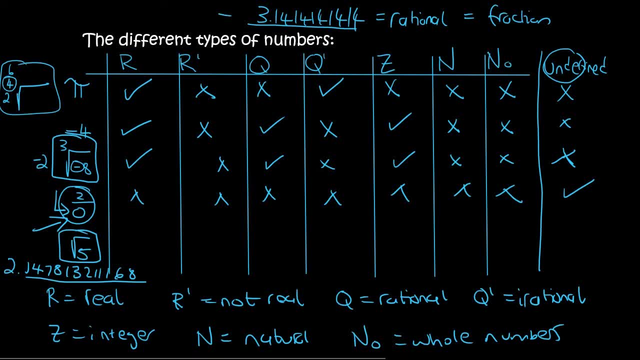 eight. So there's no pattern. The numbers are not repeating like up at the top here. So that is not going to be rational, That is irrational. But first, is it real? Yes, we can see it, Is it So? it's obviously not that one. Is it rational? No, because the digits aren't. 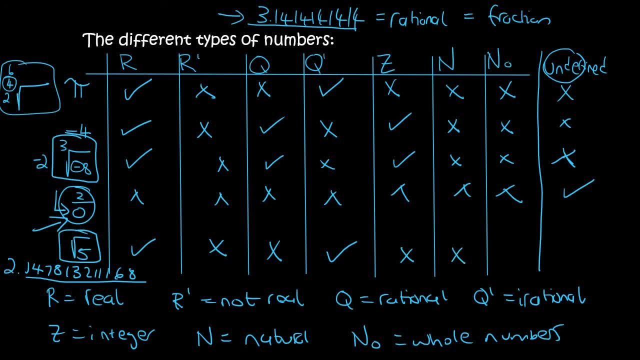 repeating. So it must be rational. It's not an integer, It's not natural, It's not a whole number and it's not undefined. And so there we have it, guys. You might have to watch this a few times just to practice, But those are the different types of numbers that you need to know. 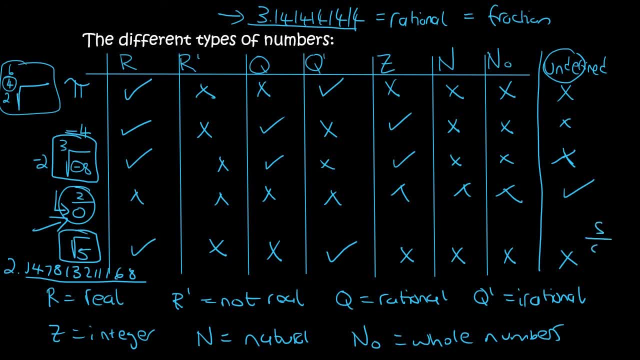 Just one more thing: Undefined is when you have a zero underneath, and nonreal is when you have an error. But when it's from a square root, then we call that nonreal. That's the only nonreal that we have, So there's only two kind of errors. When you have a zero underneath, then we call it. 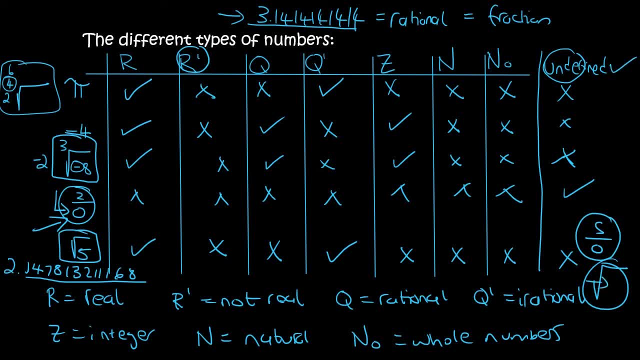 undefined, And when you have an error from a square root, then it's called nonreal, which is this one over here. Thanks for watching.